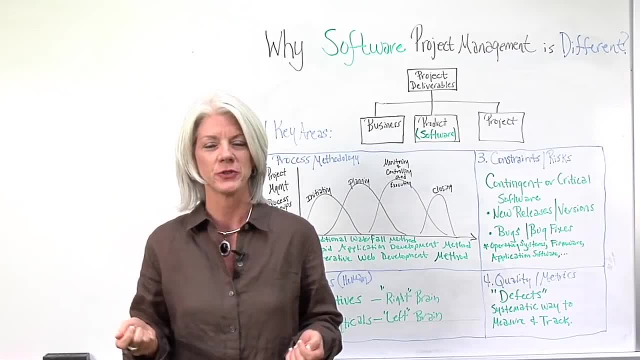 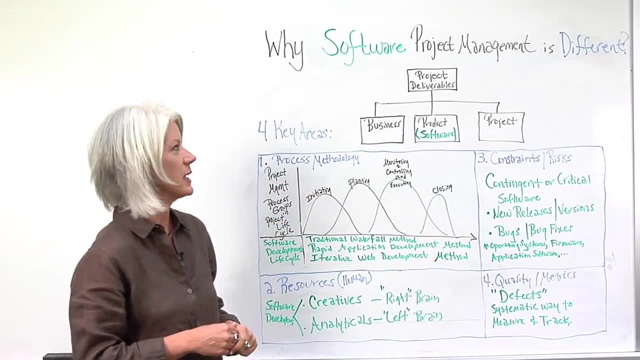 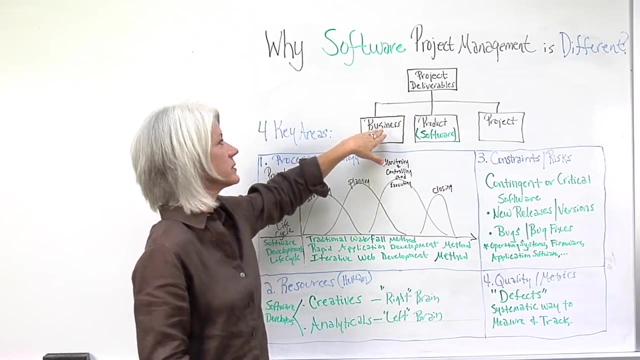 Well, there are some idiosyncrasies depending upon what industry, but today we want to focus on the software project management, And there are four key areas that we want to look at today. But I want to remind, give a reminder, that for any project, there are project deliverables where there's still business deliverables. 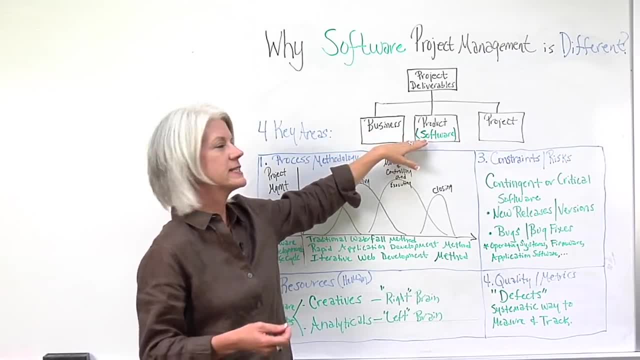 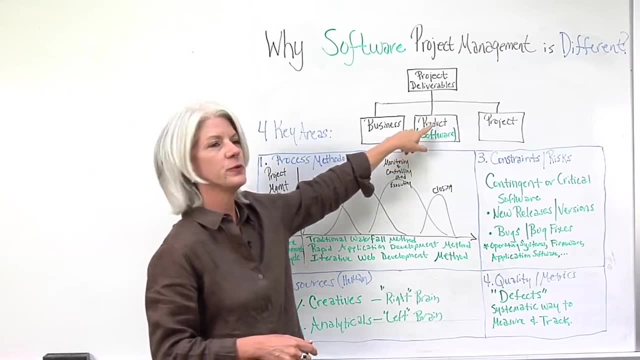 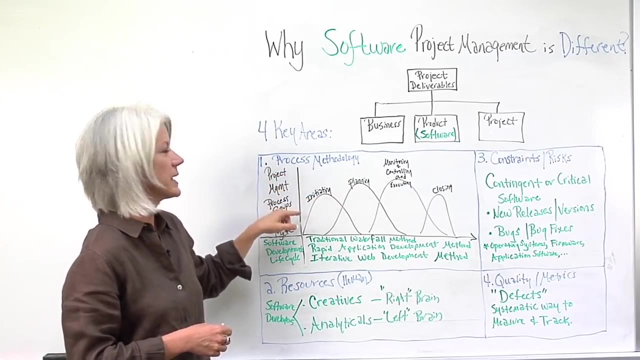 still a product or service deliverable, in this case software, and also project management deliverables. So, keeping that in mind, these are the four key areas related to the project. So, number one, the process methodology. So still, we have the project management lifecycle or process management groups in the project lifecycle. 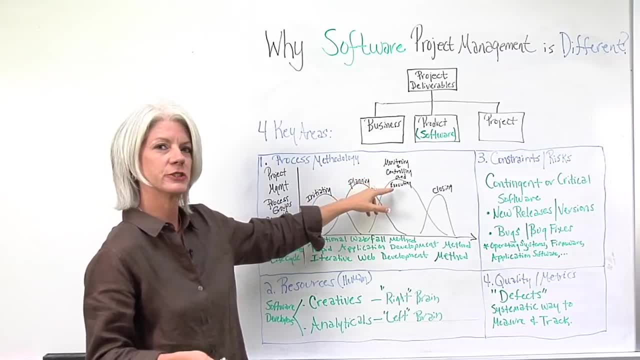 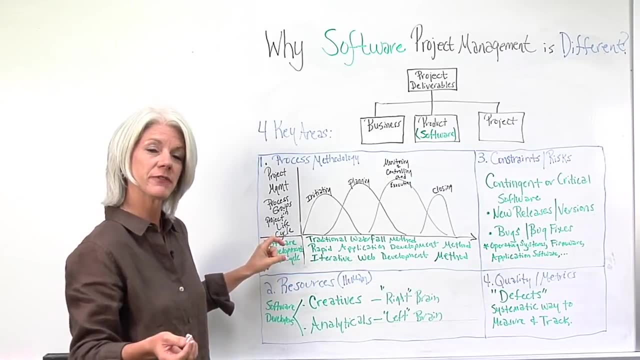 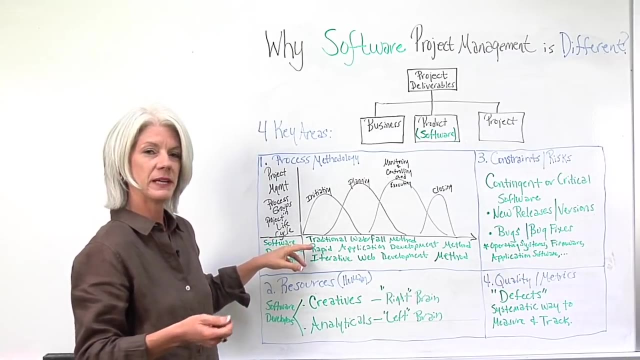 like the initiating, the planning, the monitoring and controlling and executing and the closing. And here is the bottom part, where the process methodology could be different because it depends upon the type of software development that's occurring, Some depending upon the software development or software being generated. 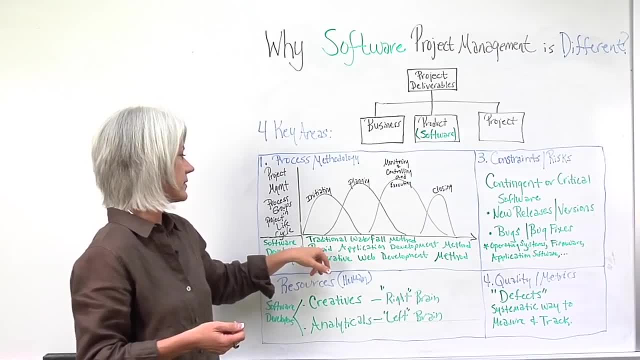 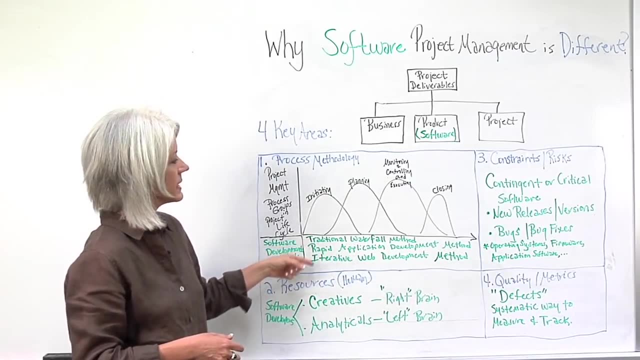 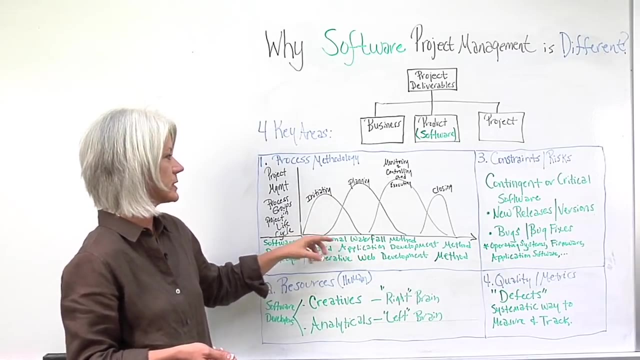 there's the traditional waterfall method, there is rapid application development method, as well as an iterative web development, and there are many more. But so in this area, depending upon what software is being generated, depends upon what process methodology is used. So this is where the change occurs. 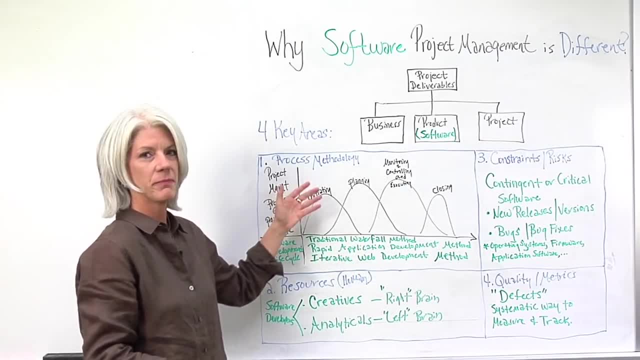 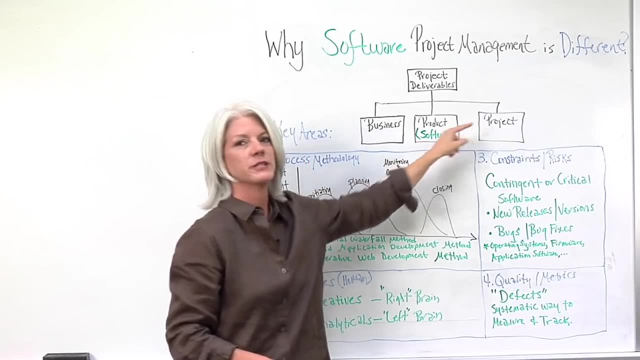 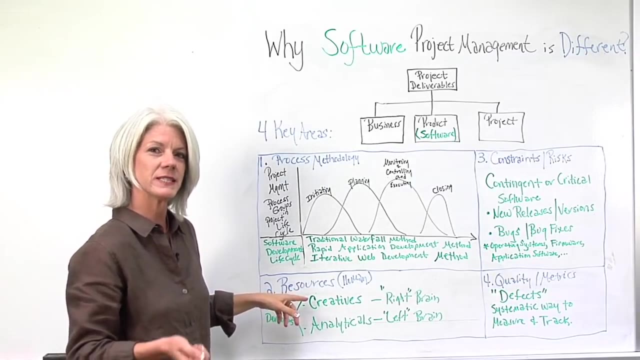 So it's the software development lifecycle, The project management lifecycle, Process groups and lifecycle is still the same because, remember, we're producing the project management deliverables here and the product or the software deliverables here. The second area are the resources. 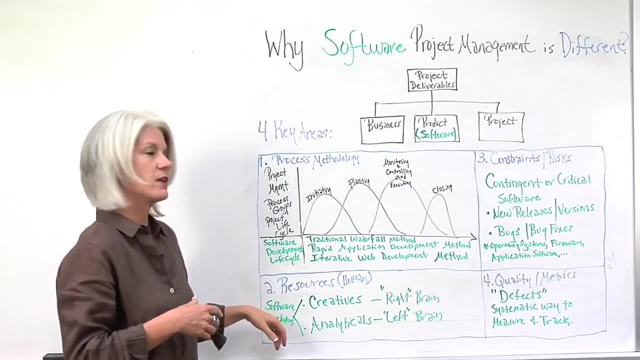 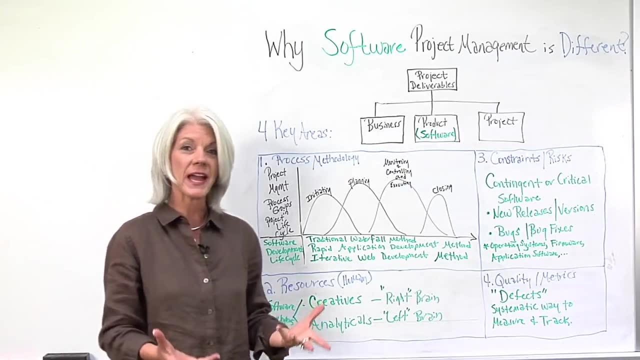 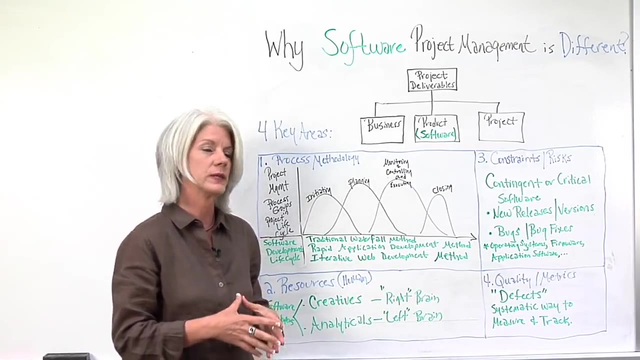 In this case, the human resources, specifically the software developers. Depending upon what type of software is being created, there are the creatives, the creative types, the right brain people, and the analyticals, the more left brain, Because, depending upon what type of software, 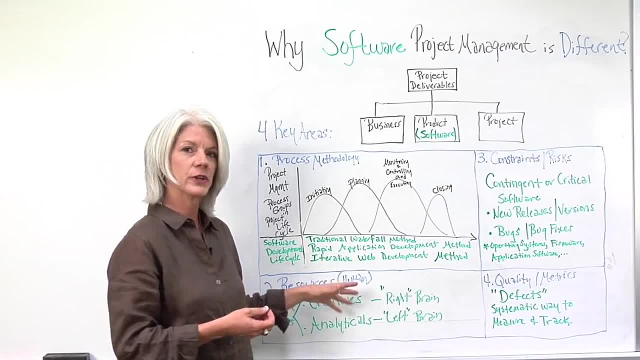 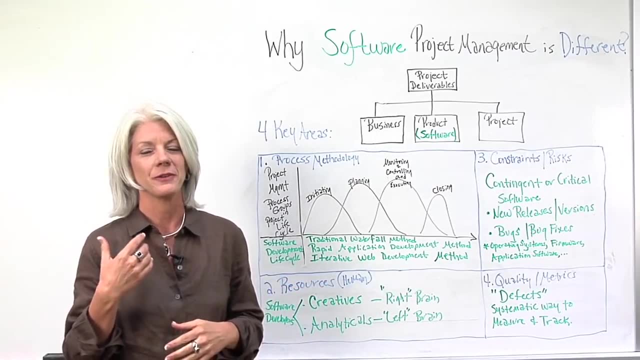 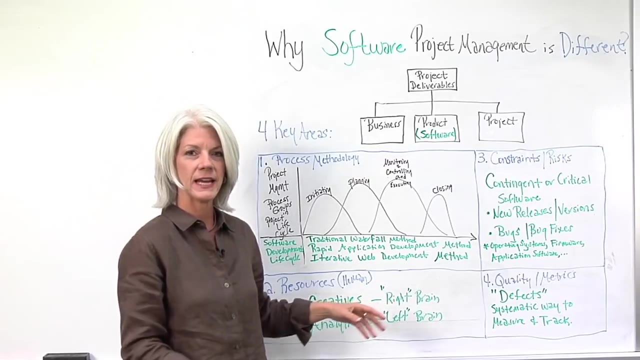 it could be more of an engineering type, or it could be graphic design, But regardless, we have the right brain and left brain resources on our project, So we manage them differently, because the creatives have to have a creative outlet They like creating.